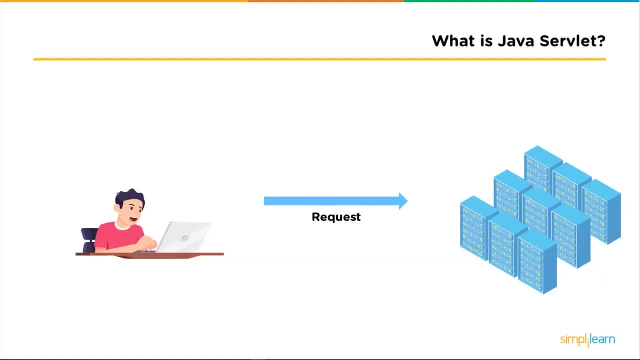 request. So further, this request is sent to the cloud or, in technical terms, your browser sends your request to the respective server responsible for storing for that particular information and helps you with it when requested. Now the server gets triggered with your request and in 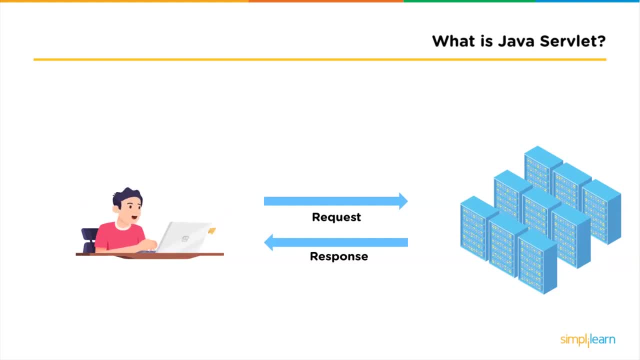 written. it helps you back with the information you have requested for. This answer from the server is called the response. So this is how the request and response work in a server. For this process to happen so smoothly, we need to start with the request and response. So let's start with the. 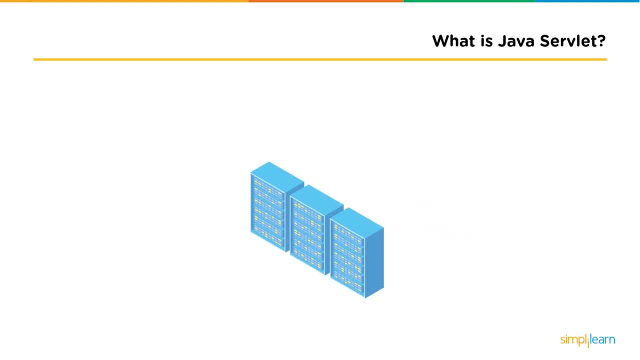 request and response. So this is how the request and response work in a server. For this process to happen so smoothly and effectively, we need a servlet. Digging a little deep into the server, we find the component responsible for such an effective job. It is called the servlet container. 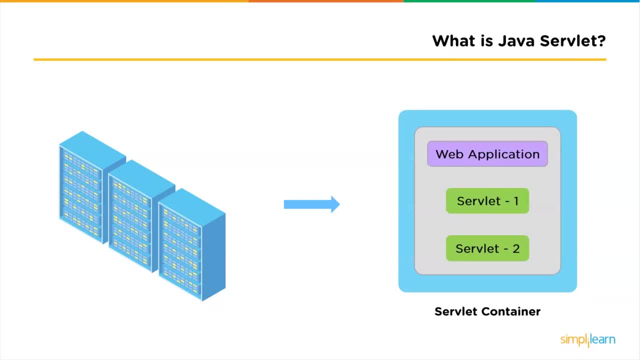 that holds Java-based web application and a set of individual components called as servlets. Now we are close to our answer. So this particular Java-based component takes care of web request and response. To sum it up with the form of a definition, we can define it as follows: 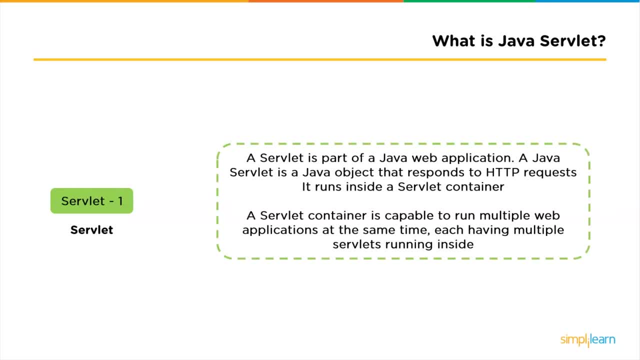 Servlet is a Java program that runs on the Java enabled web server or application server. They are used to handle the request obtained from the web server, process the request, produce the response and then send a response back to the web server. Now, hoping that it was a clear explanation, can we move ahead with the next topic? 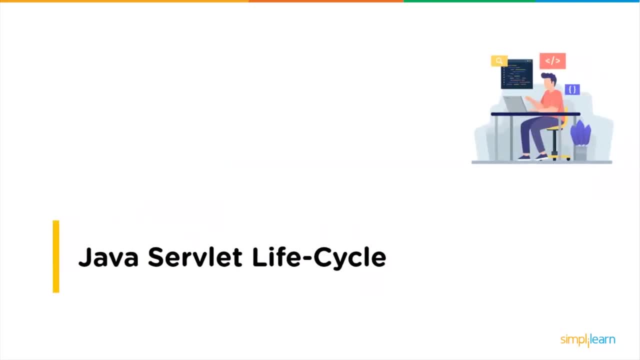 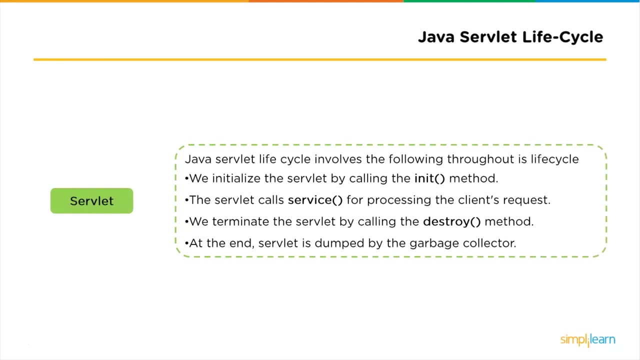 So the next topic we have is: so how does the servlet work in reality? or more practically or in depth, what's the life cycle of a servlet? So the life cycle of a servlet in real time has the following stages. These stages are the ones that a Java servlet actually follows in real life to get our work. 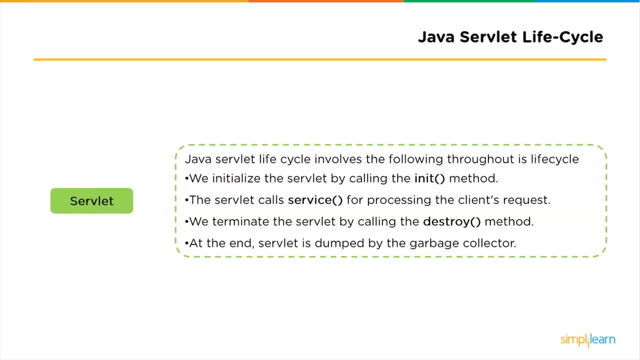 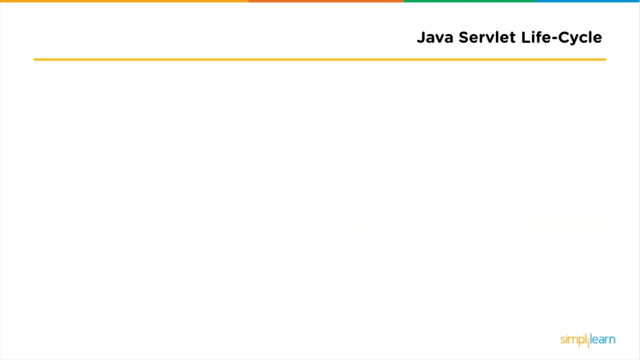 done So. the stages are init service and the CRUD operations, which are the get, post, put, delete and finally destroy. Now let us understand each one of them in a bit more detail. The first one is the init process. The init method is called only once. 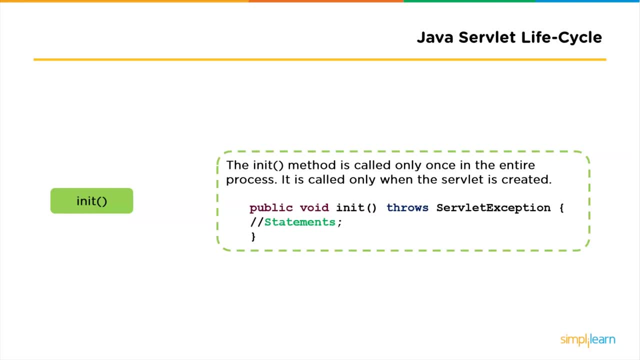 It is called only when the servlet is created and not for all the requests afterwards, So it is used for the one time initializations. just as with the init method of applets, The servlet is normally created when a user first invokes a URL corresponding to the servlet. 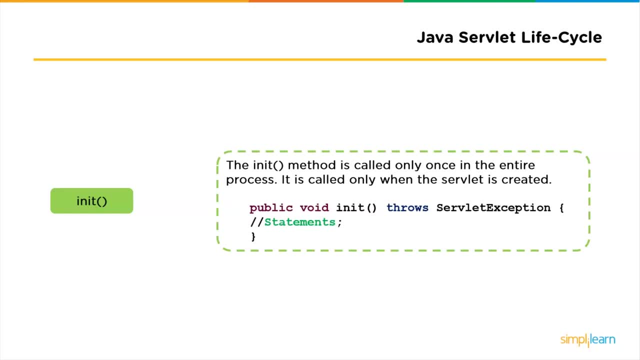 But you can also specify: the servlet is loaded when the server first started. When a user invokes a servlet, a single instance of each servlet gets created, with each user request resulting in a new thread that is handed over to the doGet or doPost, as appropriate. 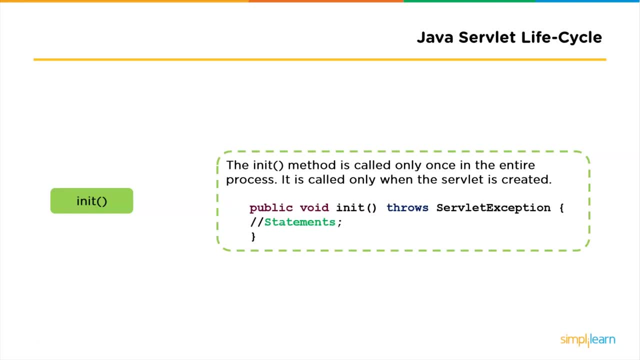 The init method simply creates or loads some data that will be used throughout the life cycle of a servlet. Followed by the init method, we have the service method. So what is service method? Service method is the main method to perform the actual task. 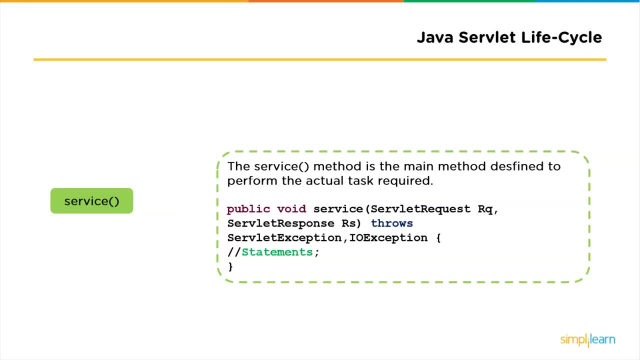 So what is service method? The servlet container, that is, the web server, calls the service method to handle requests from the client or the browser and to write the formatted response back to the client. Each time the server receives a request from the servlet, the server spawns a new thread. 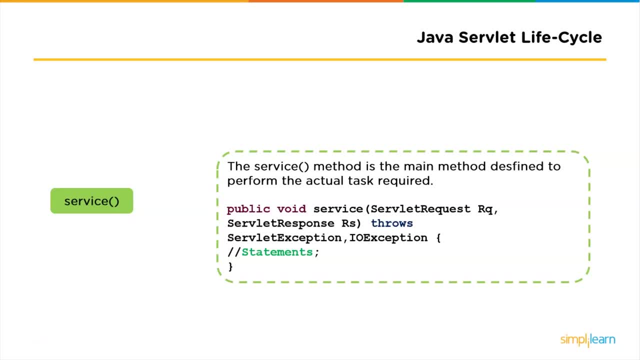 and calls service. The service method checks the HTTP service type and accordingly performs the CRUD operations, which are the get, post, put, delete, etc. And calls doGet, doPost, doPut, doDelete, etc. methods as appropriate. The service method is called by the container and service method invokes doGet, doPost, doPut. 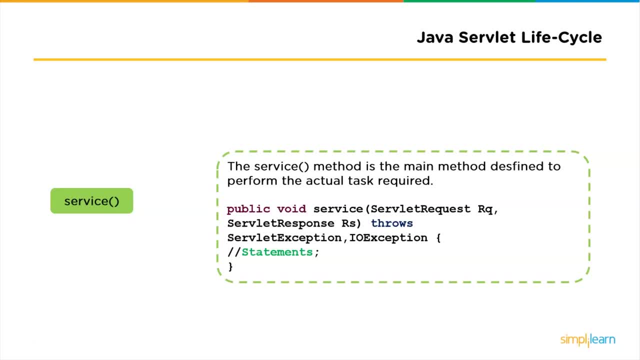 and doDelete etc. methods as appropriate. So you have nothing to do with service method, but you override either with doGet, doPost and other types, depending on what type of request you receive from the client. So this is how the init method works. 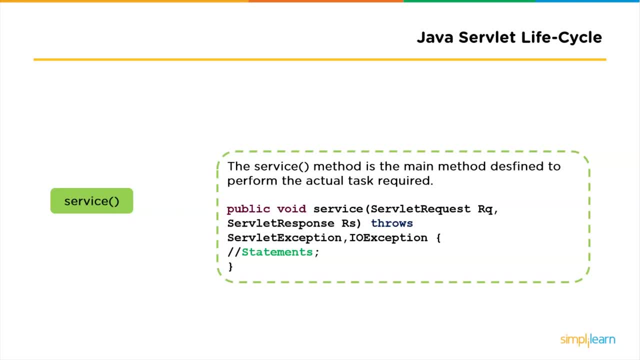 So this is how the init method works And service methods work. Now, digging a little deeper, we have the doGet, doPost, doDelete and doPut methods. So first we will discuss about doGet method. So what exactly does a doGet method do? 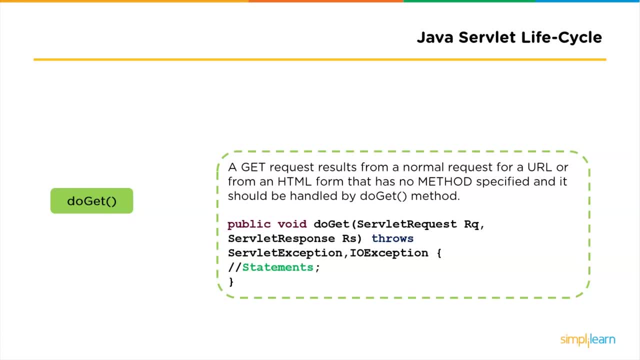 A get request results from a normal request, from a URL or an HTML form that has no method specified and it should be hardly by doGet method followed by doGet. We have doPost. A doPost request results from a HTML form that specifies list post as the method and 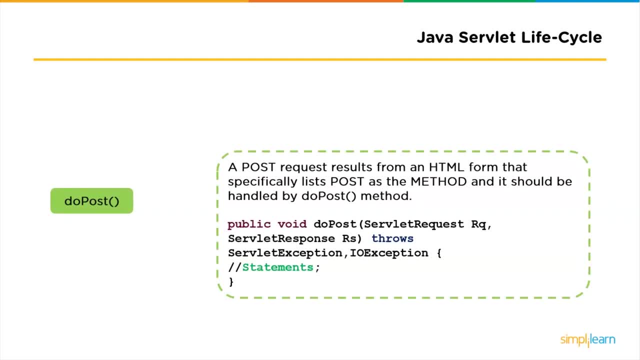 it should be handled by do post method Similar to doGet and doPost. The doput and doDelete options are usually used to update and delete the data when asked by the client. So to sum up these doGet, doPost, doPent and doDelete, we can consider them as CRUD. 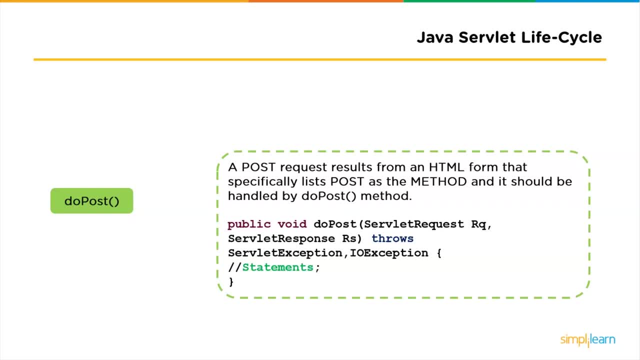 operations. So doGet basically gets the information what you're looking for. DoPера makes it personal and private method usually posts the information or provides you with the response from the server and followed by that we have the do put, which is usually used to update. 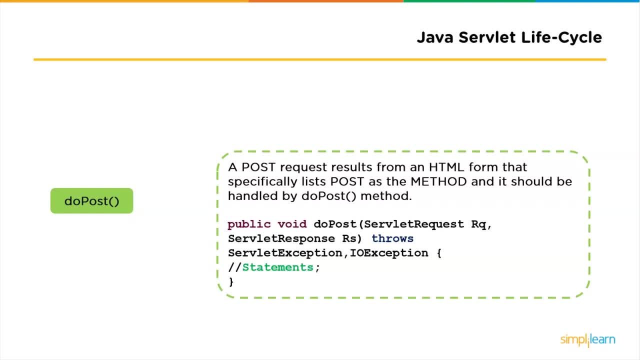 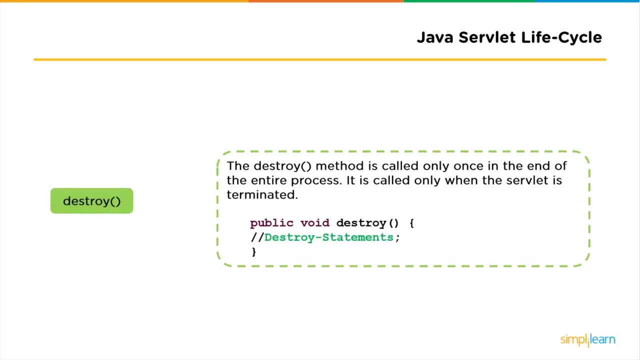 the data which is present on your server and finally delete, which is used to delete an existing data on your server. so this can be considered as CRUD operations. and finally we arrive at the last method, which is the destroy method. the destroy method is called only once, at the end of the life cycle of a. 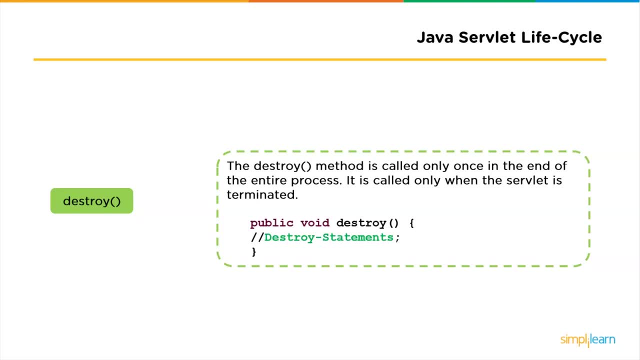 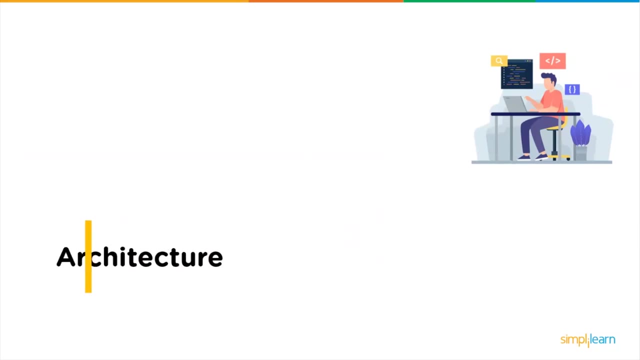 servlet. this method gives your servlet a chance to close database connections, halt background threads, write cookie list or hit counts to the disk and performs other such cleanup activities. so with this we finish up the life cycle of a servlet. now we shall understand its architecture. basically, the architecture of a servlet can be understood by reverse engineering. 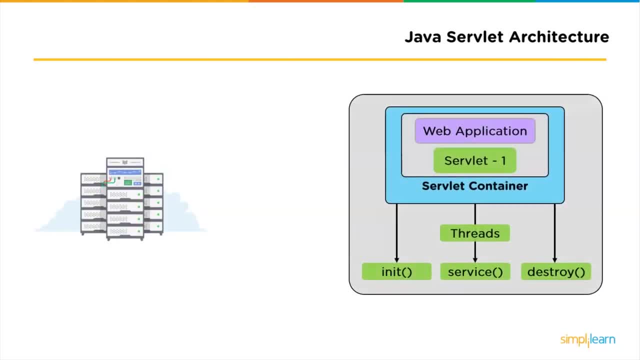 the life cycle of a servlet. so this is how the servlet execution takes place when a client or a browser makes a request to the web browser. so the servlet architecture includes the following: first one servlet interface. to write a servlet, we need to implement the servlet interface. servlet interface can be implemented directly or indirectly by: 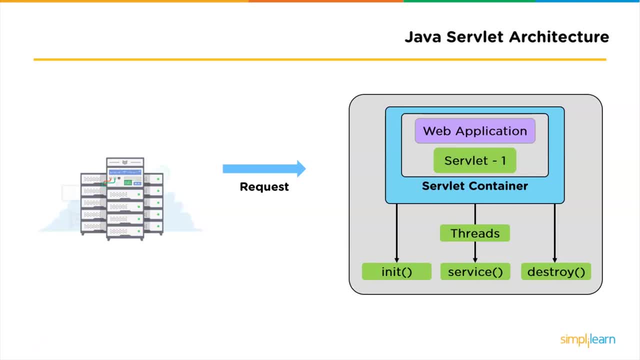 extending generic servlet or HTTP servlet class, followed by that. the next part is request handling methods. as we have discussed before, there are many, mainly three, methods defined in servlet interface, which are in it service and destroy, and inside service. we have do put, do post, do get and do delete methods. the 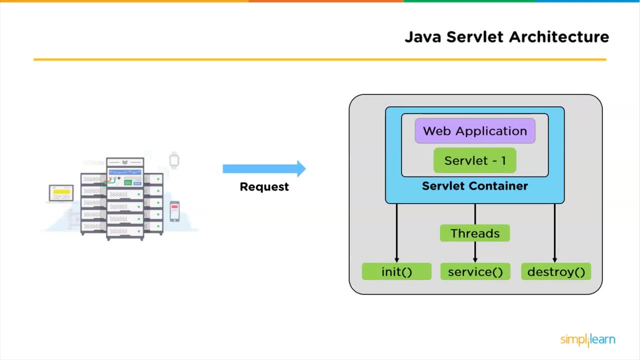 first time a servlet is invoked, the init method is called. it is called only once during the lifecycle of a servlet, so we can put all your initialization code here. the service method is used for handling the client request. as the client request reaches the container, it creates a thread of servlet object, and request and response object are also. 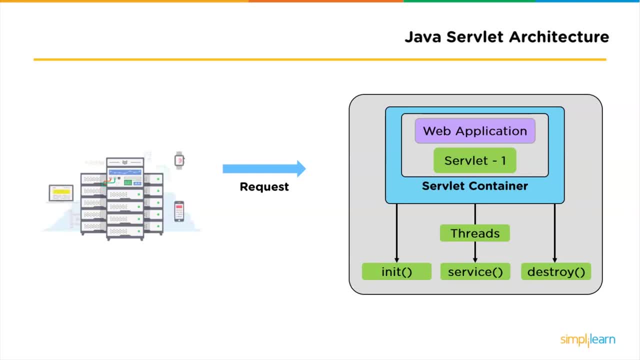 created. these request and response objects are then passed as parameter to the service method, which then processes the client request. the service method in turn calls the do get, do post methods, if the user has extended the class from HTTP servlet. and, lastly, the creation of instances. this is based on the load of 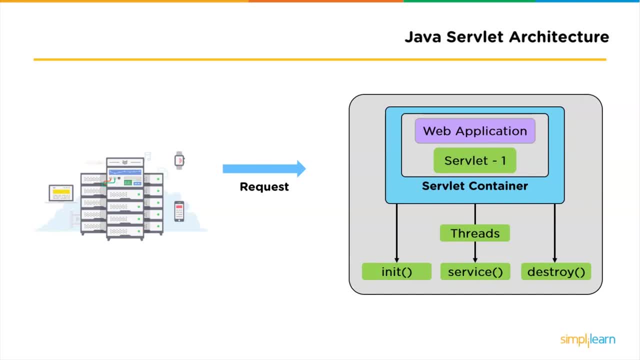 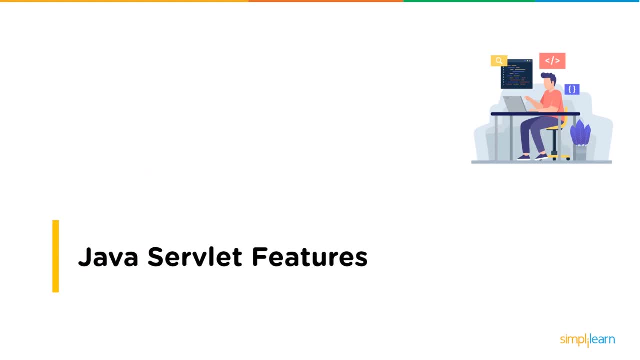 the servlet. so with this we have finished the feature of servlet. moving further, we shall quickly discuss the features of servlets and then enter into the practical mode. so the following are the features of Java servlets. the first feature is Java. servlets are portable in nature. as I have mentioned above, the servlets use Java as 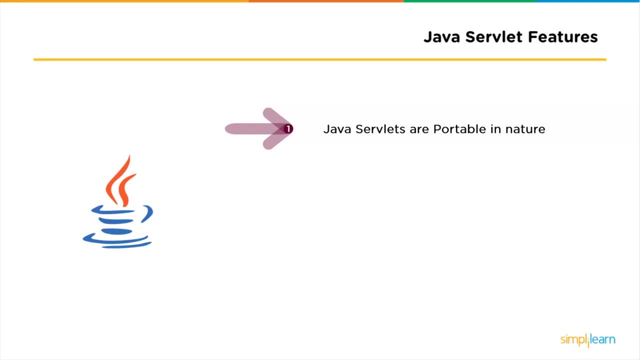 programming language, since Java is a platform independent programming language. the same holds true for servlets. for example, you can create a servlet on Windows operating system that uses glassfish as a web server and then later run it on any operating system like Unix, Linux and Apache Tomcat web server. this feature makes servlet portable, and this is the main advantage of servlet. 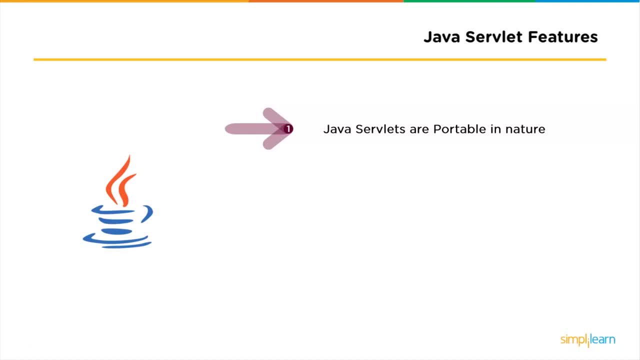 over CGI. we shall discuss all the differences of CGI versus servlet in the next section. for now we will discuss the features. first feature. we will now enter into the second feature, which says Java servlets are efficient and scalable. once a servlet is deployed and loaded onto a web server, it can instantly start fulfilling the 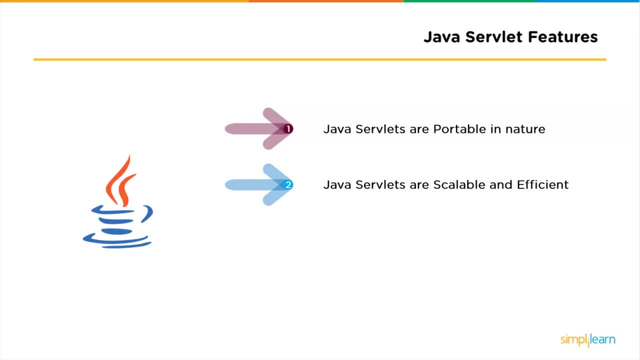 request of the clients, the web server invokes servlet using lightweight thread, so multiple client requests can be fulfilled by servlet at the same time, using the multi-threading feature of Java. compared to CGI, where the server has to initiate a new process for every client request, the servlet is truly efficient and scalable. the next and the final feature of Java. 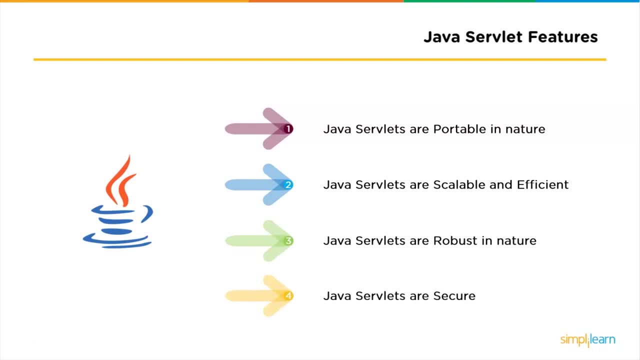 servlets is they are robust and highly secure. by inheriting the top features of Java, such as garbage collector, exception handling, Java security manager, Etc. the servlet is less prone to memory management issues and memory leaks. this makes the development of web applications and servlets secure and less. 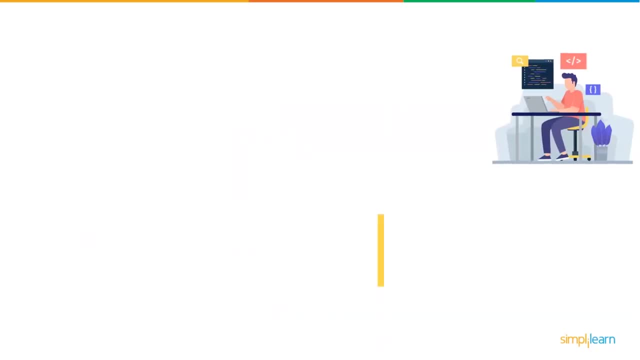 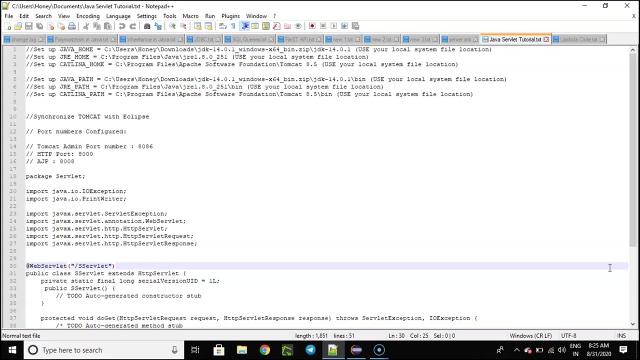 error-prone. so these were the important features of Java servlets. now let us enter the practical mode. so we are in the practical mode right now. there were two parts in the practical mode. the first one was to set up the environment for Java servlets and the second one was to execute a basic program. 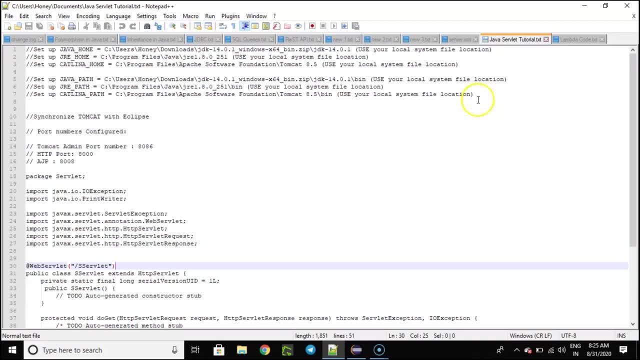 so this document has the following steps to follow, that is, the prerequisites, before executing a Java servlet program. so we have these prerequisites, where we have to set up Java home and Java path. followed by that we need to set up the home and path for JRE, which is the Java runtime environment, and finally Catalina home and path. so Catalina home. 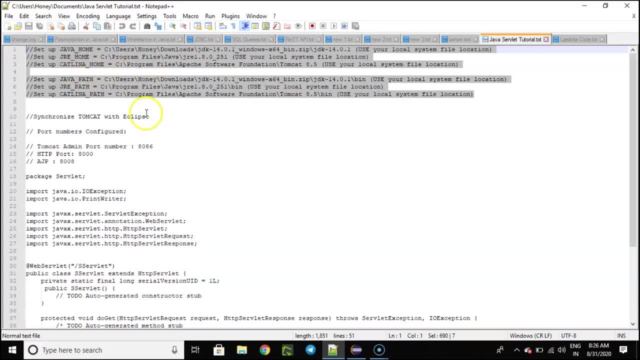 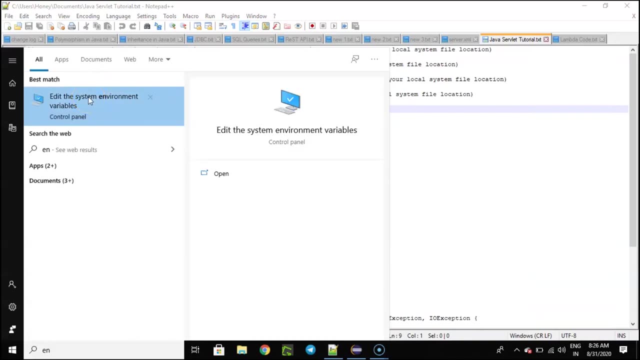 and path is nothing but the tomcat server home and path. now we will set up these things by using the environment variables. now I'm using a Windows operating system, so I'll be using the control panel to enter the environment variables. there you go. you have edit environment variables, so inside that, just select environment variables. 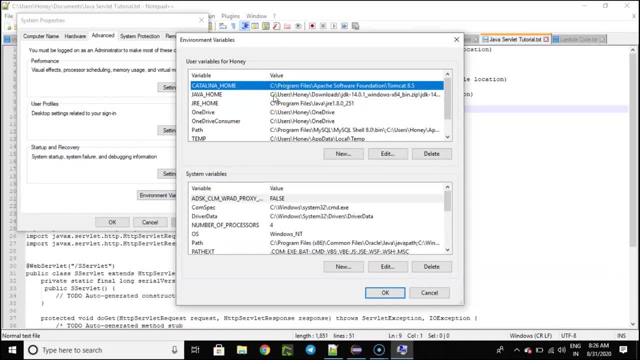 and inside this you can see that I have already set up the environment variables for Catalina home, Java home and JRE home. so now let us just select Java home and edit it so that we can see: how did I set it. so you can see I have named the variable name as Java home. 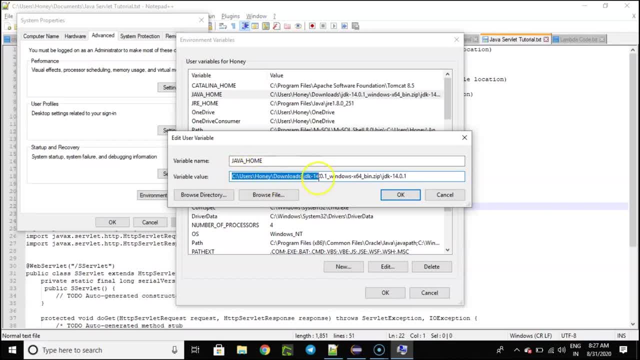 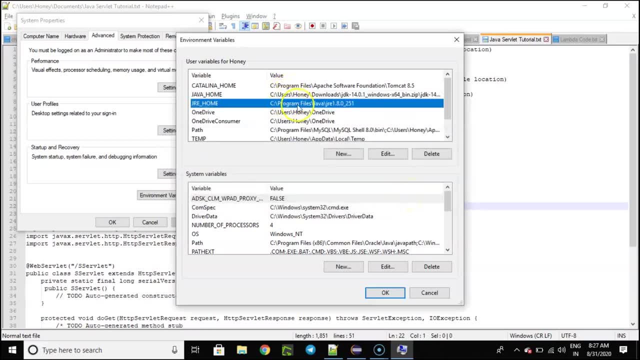 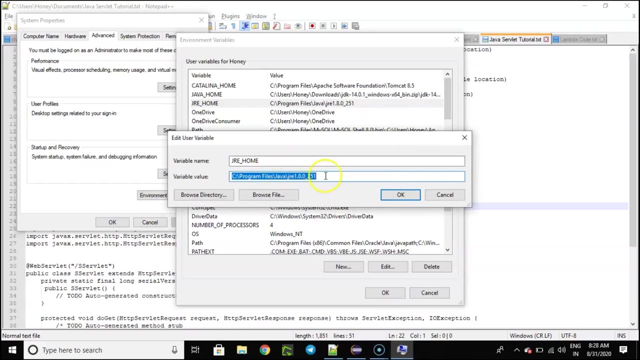 and inside the variable value I have a location. so this location is nothing but the Java JDK location in my local system. now, followed by that, we have JRE home, so similar to Java home, we have set up the JRE home as variable name is equals to JRE home and the variable value is the location of. 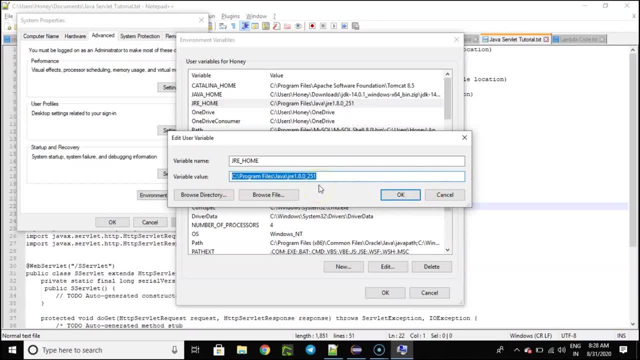 JRE folder in my local system. so I have my JRE folder in my local system at C drive program files, the Catalina home which is inside my program files, Apache, software foundation and tomcat 8.5. so similarly we'll also check up the path variables. so inside system variables you can. 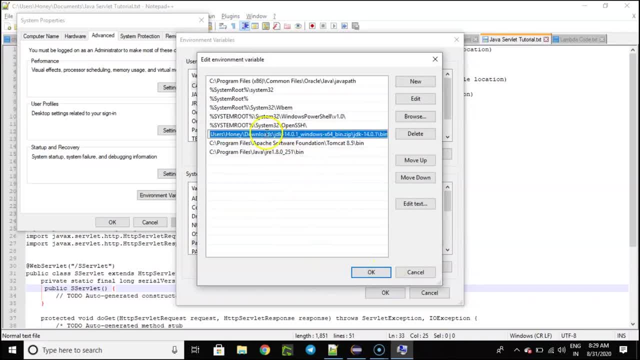 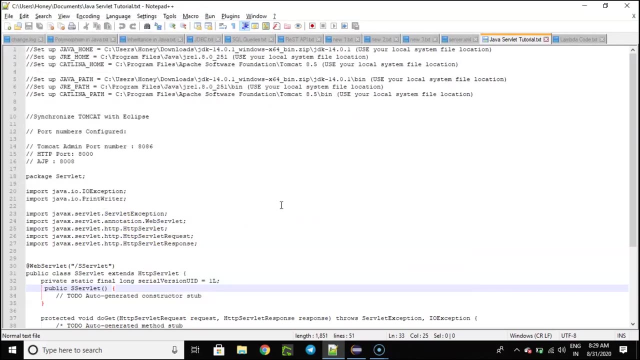 see the path, just edit it so then you can see the path variables set for Java, JRE and tomcat. now just select okay, okay and finally another okay. requisites have been set up. so this is how you set them. so in case, if you have doubts about the Tomcat version to download, then I'll help you with that. 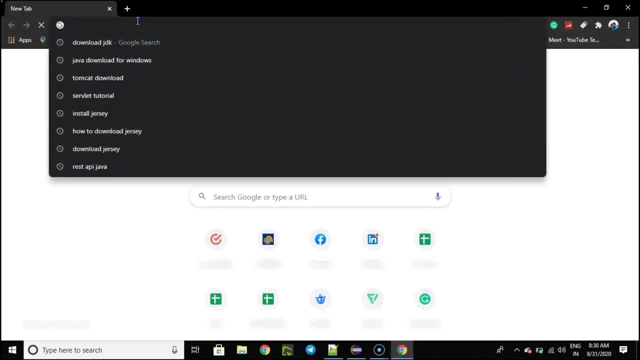 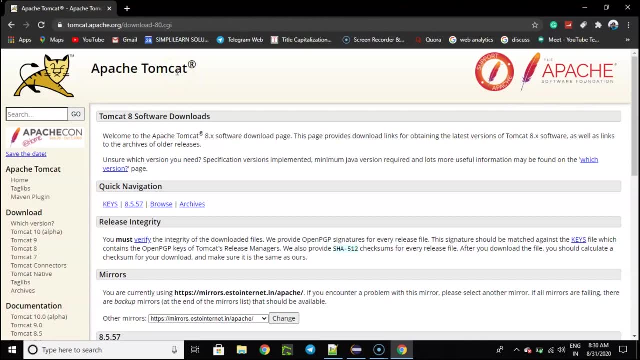 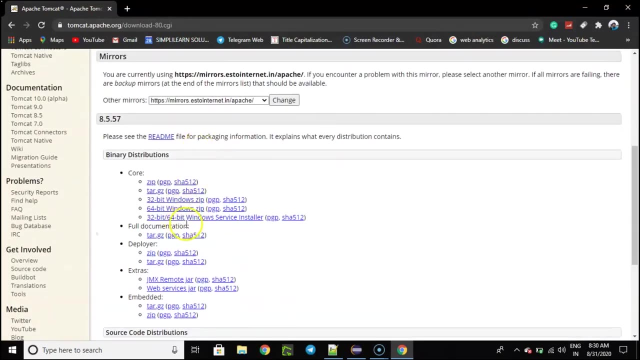 just open Google and type in Tomcat download. so now you have entered Apache Tomcat official site and since I'm using a Windows operating system, I'll be selecting the 32-bit or 64-bit a Windows service installer version and after this gets downloaded, you need to set up. 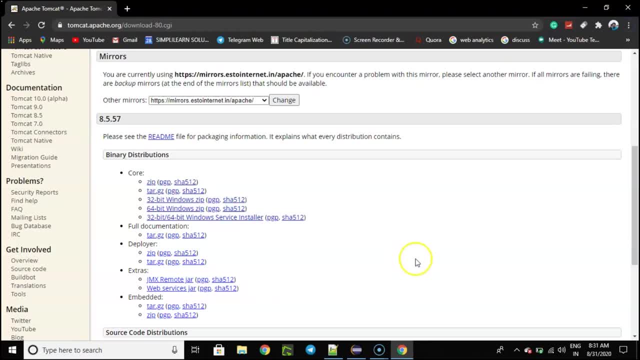 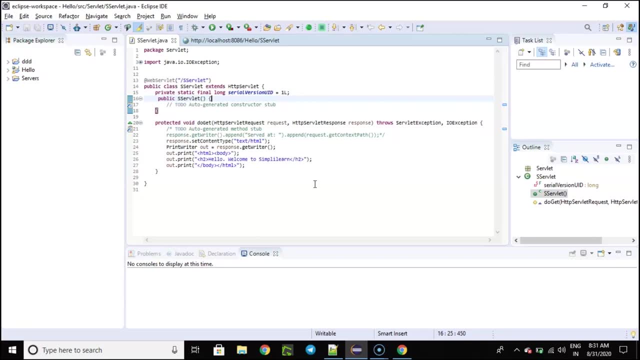 the home and path variables for Catalina server. so once after the environment is set up, you need to follow four stages to create a servlet program, which are creating a dynamic web project: create a servlet, add servlet API jar file and run the servlet. so to create a dynamic web project, you 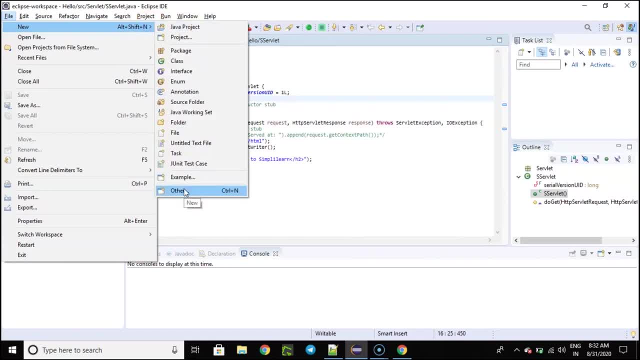 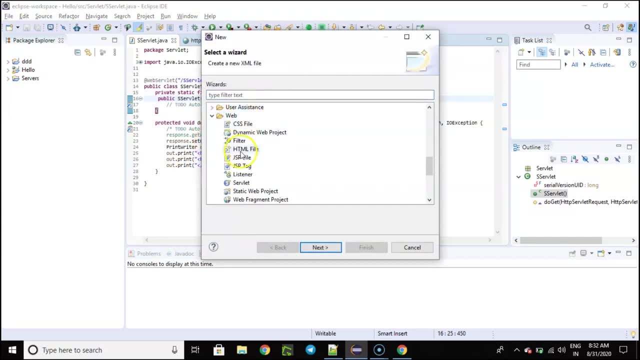 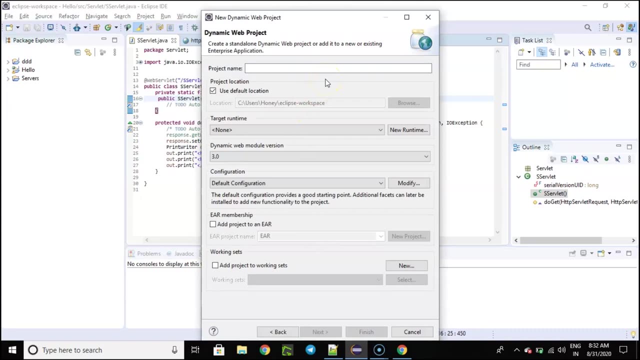 need to select new and inside that you have the option of other. just select other and inside that you'll be finding web. so select web and inside that you need to select the dynamic web project and select next. so you just need to name to your dynamic web project. so I'll be naming a server and then select next and 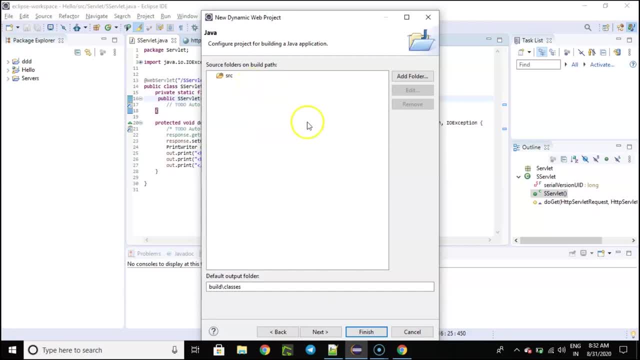 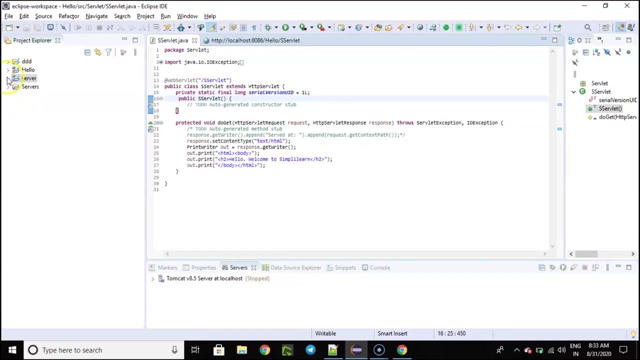 inside that you have a source folder and now you can select finish. now there you go. Java Eclipse will ask you for opening this particular in Java EE perspective. then just select open perspective. now, basically, Java will set up everything you need here and there you go. you can see server folder here, which has already. 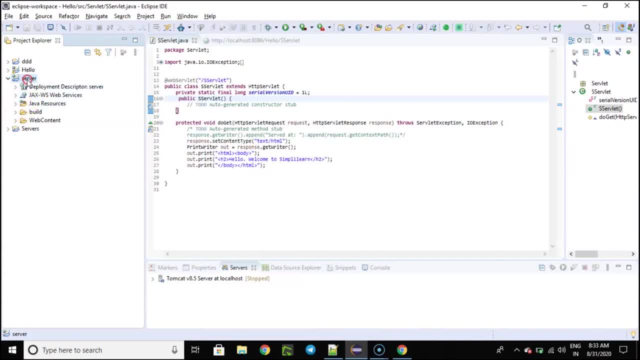 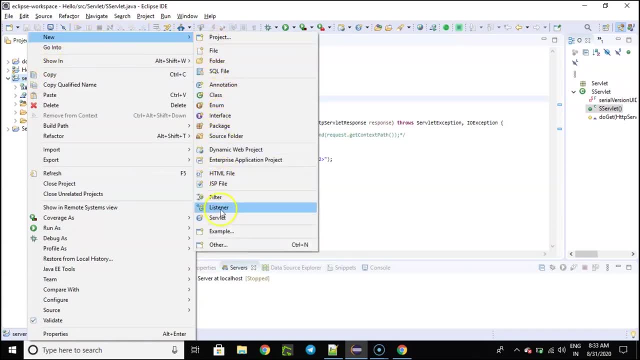 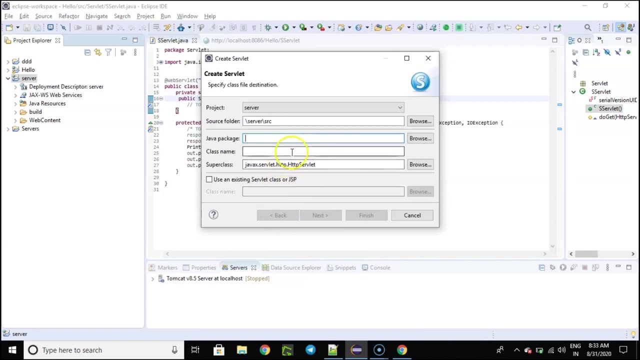 set up everything you need. now. what you need to do is set up a new servlet. so right click this and select new, and inside that you can see the option of servlet. just select it. now you can see a new dialog box and here you need to set up the class name. 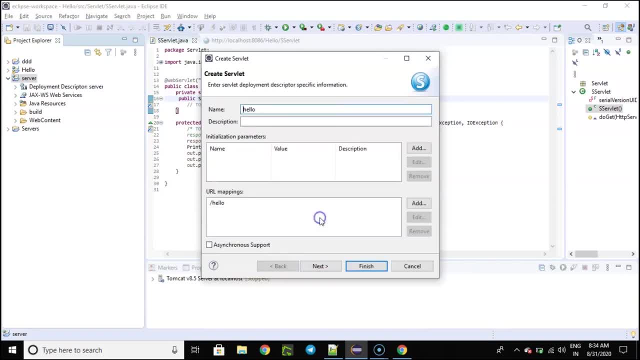 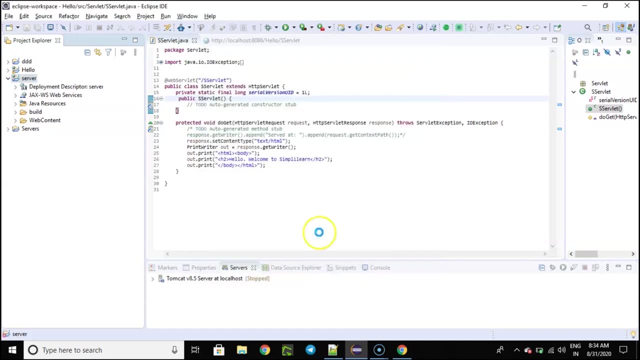 for now let's just type in hello and go to next, now again next, and in here you have a lot of options. so for now we are just executing a basic program. so let's just select do get method. now let's just finish it and there you go, your servlet. 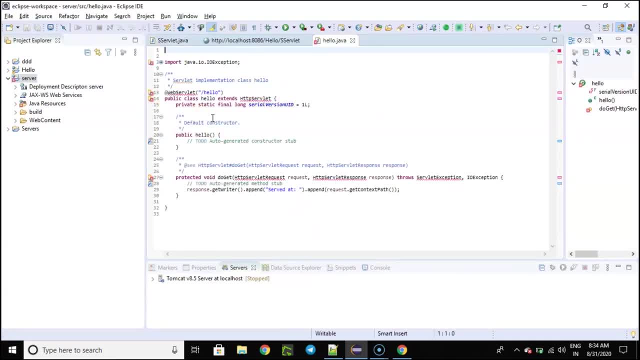 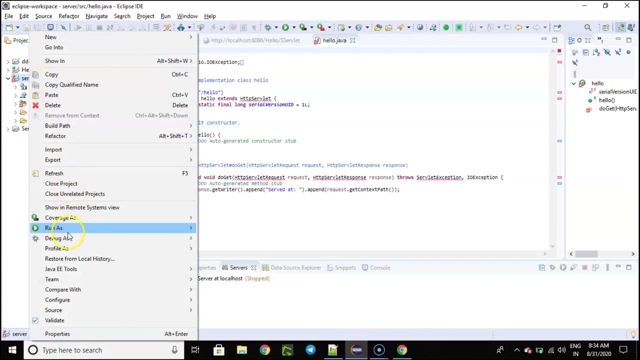 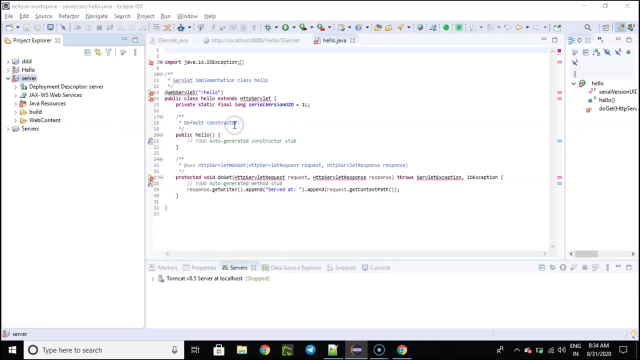 has been ready. so this is the basic template created by eclipse for you now. next we need to add in the build path. so for that you need to right click the server and then select build path and here configure build path. from here you can add the external. 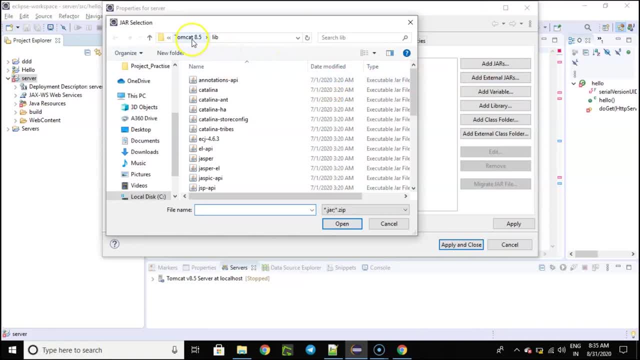 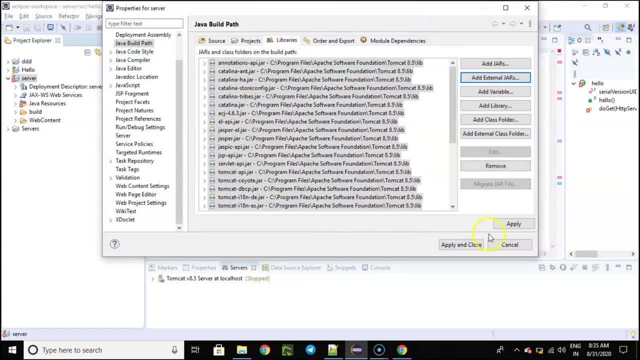 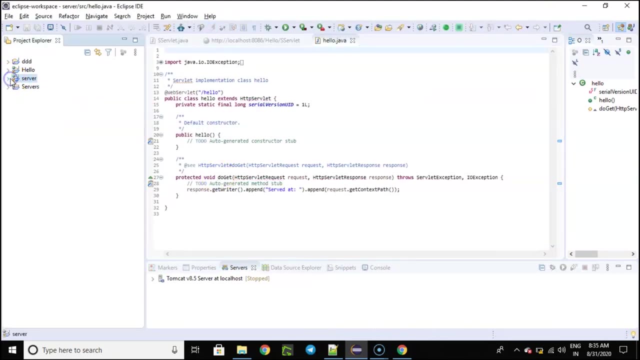 library, select the external libraries option and you can see. I have the tomcat libraries here. just select all and open, and that's how you add all the required libraries of tomcat server now apply. and now the last step is to execute the project now. just to save time, I have already typed in the program. 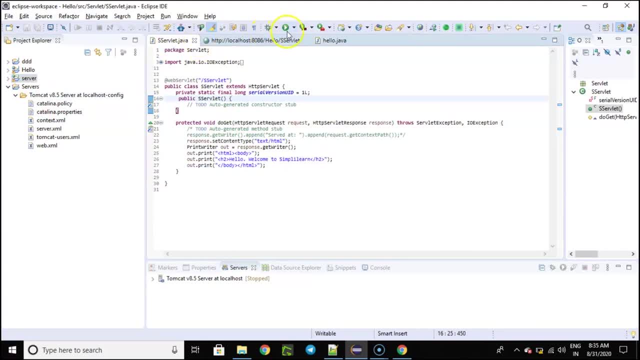 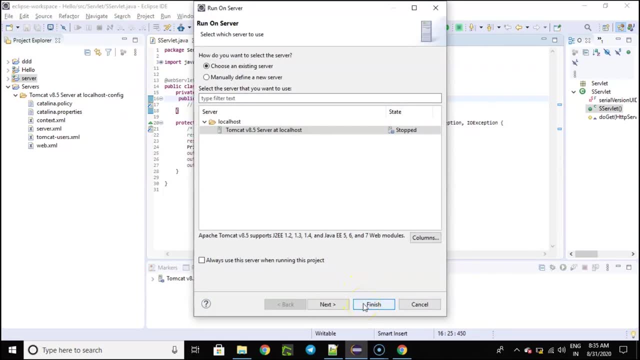 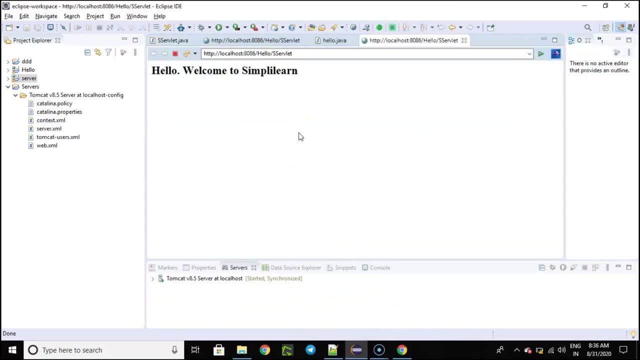 which is over here. now let's try to execute this. this program will just provide us a simple output which is none other than hello world. now the server I have, choose this tomcat server. let's finish it. so there you go. the message has been displayed successfully. hello welcome to simply live. 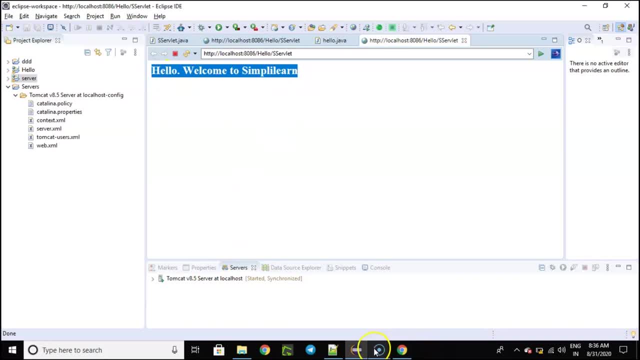 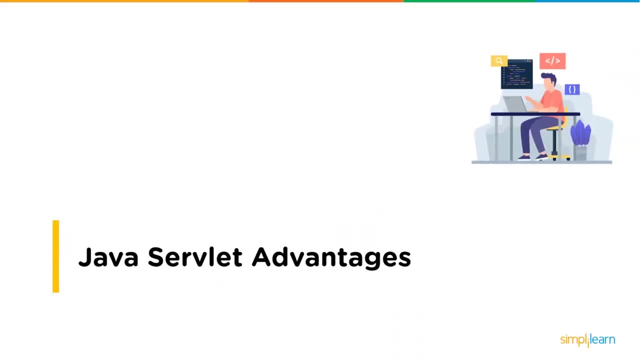 alone. now we'll move ahead with our next topic. now that we are done with the environment setup and the basic example, let us now discuss the advantages and disadvantages of using Java servlets. so first we will discuss the advantages. the following are the advantages of using servlets: 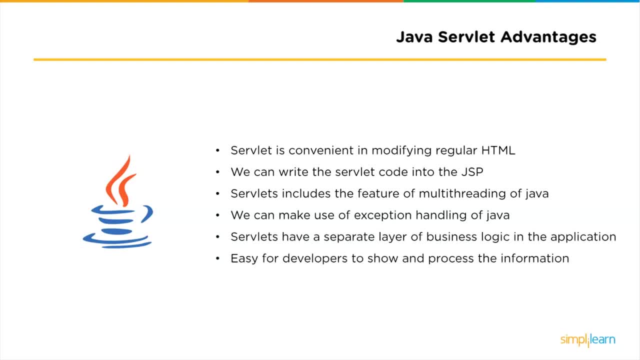 in Java servlet is convenient in modifying regular HTML. we can write the servlet code into PHP. servlets include the feature of multi-threading of Java. we can make use of exception handling of Java. servlets have a separate layer for business logic in the application and finally, it is easy. 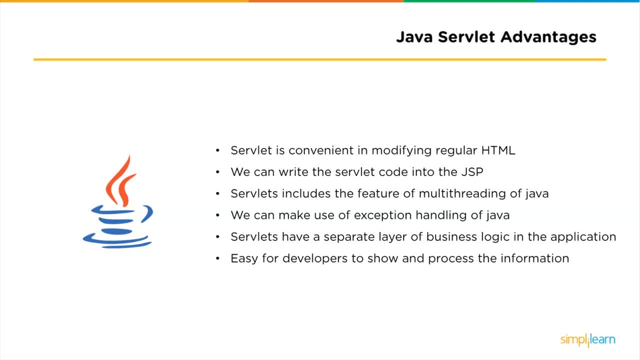 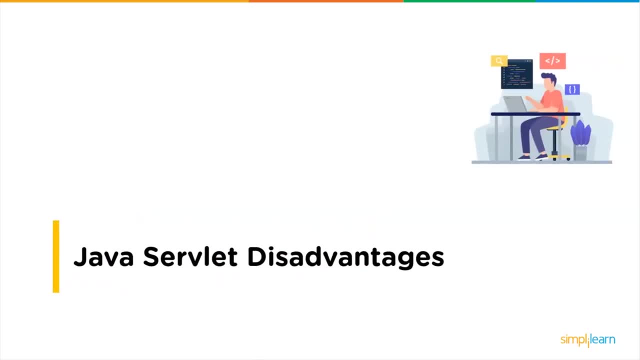 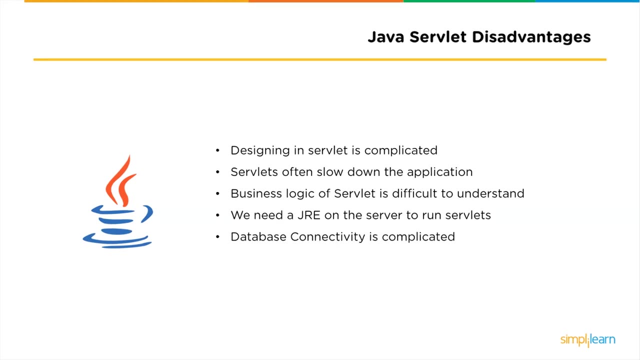 for developers to show and process the information. so these were the advantages of using servlets in Java. moving ahead, we will discuss the disadvantages of using servlets. so following are the disadvantages of using servlets in Java. designing a servlet is considered as a little complicated. servlets often slow down the application. 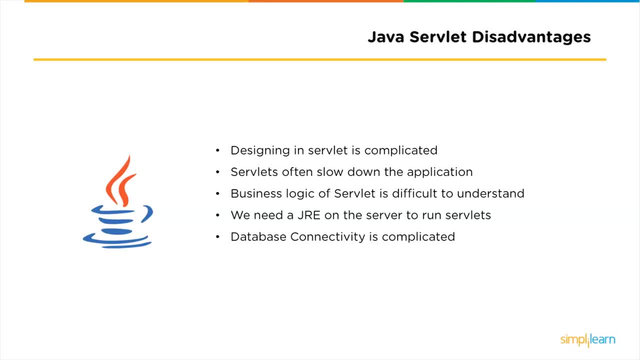 business logic of servlet is difficult to understand. we need a JRE, which is the Java runtime environment, on the server to run our servlets and finally, the data connectivity is a little complicated. so these were the major disadvantages of using servlets in Java. moving ahead, we will. 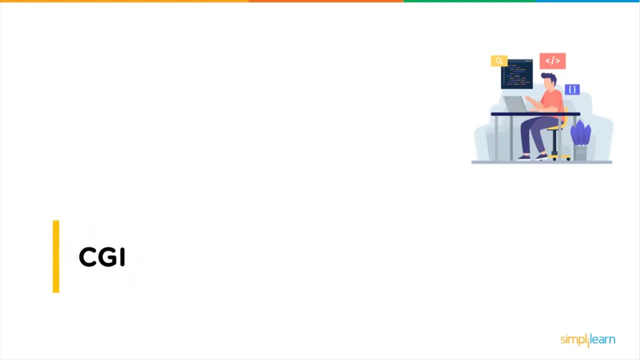 understand CGI. why are we learning CGI? because even CGI is similar to servlets and it also does the web interactive jobs similar to servlets, so thought you should know about some basics of it. so let's understand its definition and architecture real quick. so the CGI, or common Gateway interface, is a standard for writing. 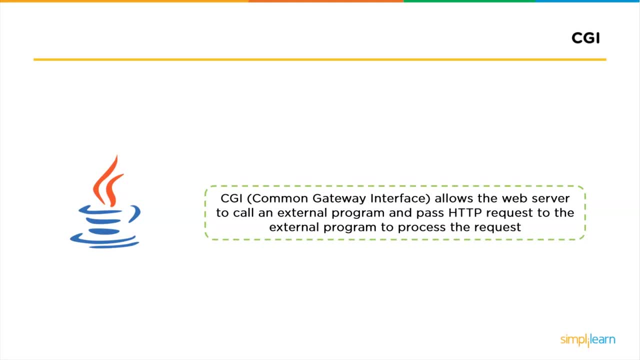 programs that can interact through a web server with a client running on web browser. these programs allow a web developer to deliver dynamic information, usually in the form of an HTML, via the browser. a CGI program can be written in any language, including Java, that can be executed by your web server. CGI programs are commonly used to add search engines. guestbook. 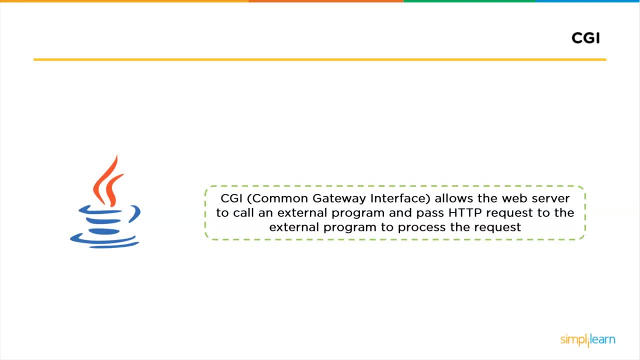 applications, database query engines, interactive user forums and other interactive applications to websites. in very basic terms, a CGI program must interpret the information sent to it, process the information in the same way and generate response that will be sent back to the client. most of the input of CGI program is passed into through. 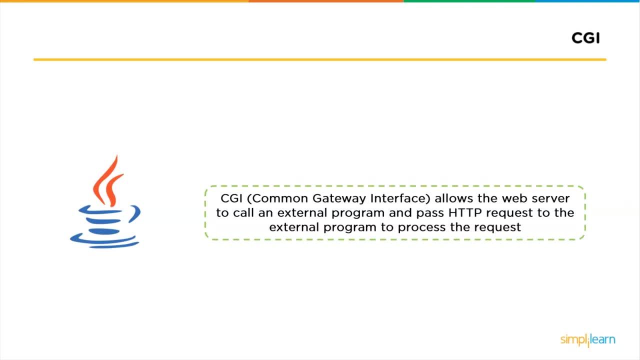 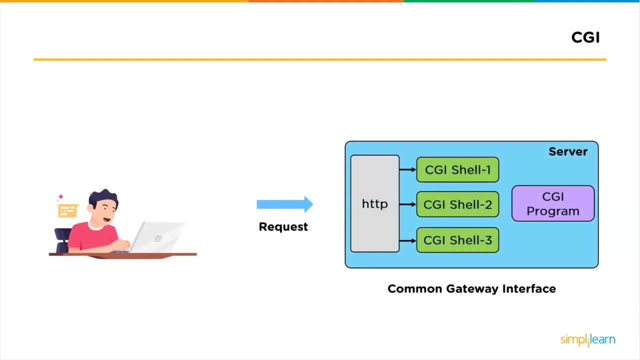 environment variables. so with this we will move ahead into the architecture of common Gateway interface. so you can see, the architecture of common Gateway interface is completely similar to servlet. normally the request is sent in the form of an HTTP request, so this particular HTTP request is divided amongst the CGI shells and it will be 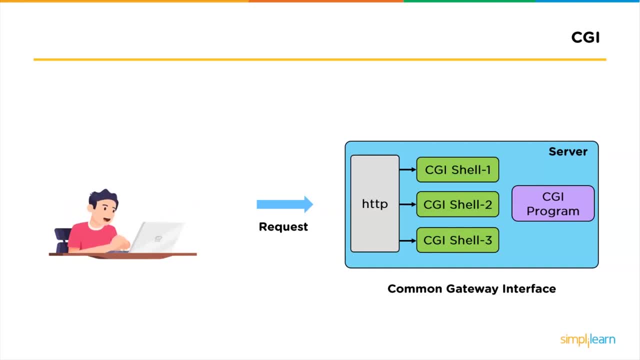 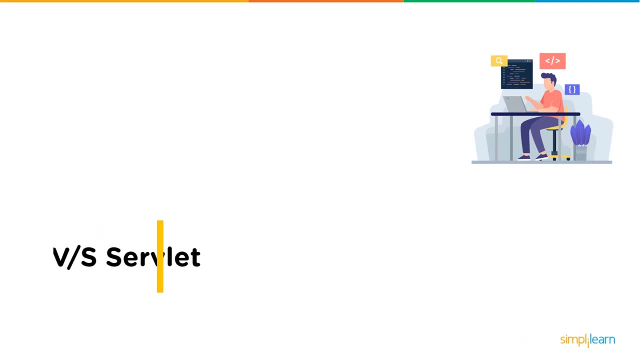 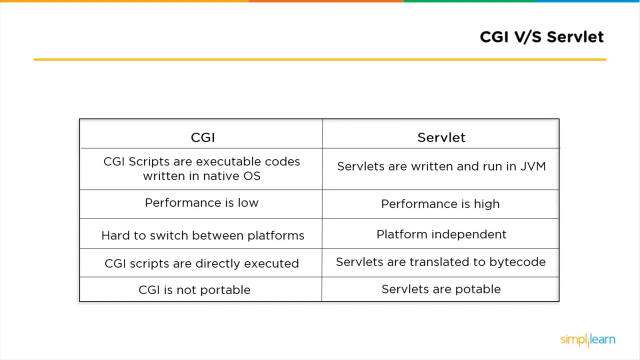 processed by the CGI shells based on the program provided, and the response is sent to the user. now, moving ahead, we shall understand the differences between the common Gateway interfaces and the servlet. so the first difference is the common Gateway interface. scripts are executable codes written in native operating system, while, on the other hand, the servlets are written and run using. 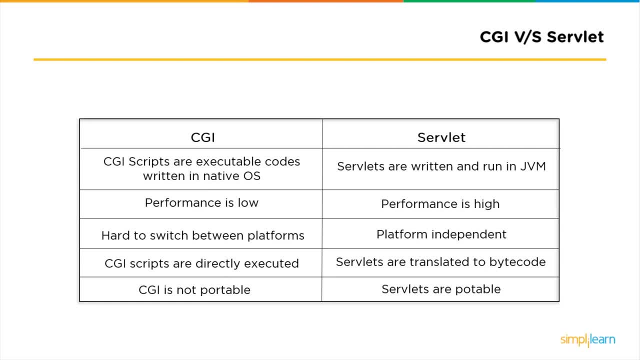 the Java virtual machine. the next difference is the common Gateway interface. performance is considered to be low compared to servets. on the other hand, servlets are having high performance compared to CGI. the third difference is, for a common Gateway interface, it is hard to switch between different platforms, that is, the operating system platforms. when we come into servlets, the servlets. 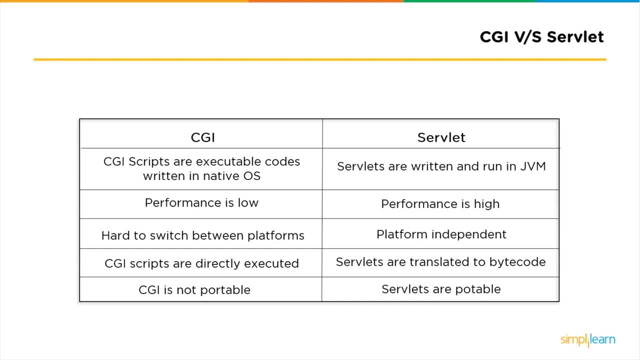 are considered to be completely platform independent, followed by that, the common Gateway interface scripts are directly executed. so hand servlets are translated into bytecode because the servlets are executed using the java virtual machine. and in java virtual machine, whatever the code you transfer, it will be converted into bytecode first, then executed. and the last difference is the common gateway. 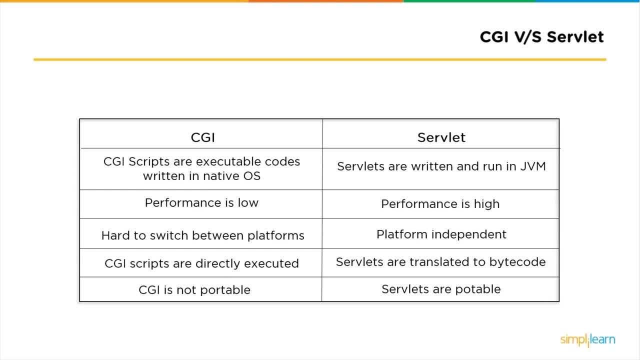 interface is not portable and on the other hand, we have the java servlets to be completely portable. so these are the major differences between the common gateway interface and java servlets. now let us understand the java servlets: requests and responses. so first we will deal with 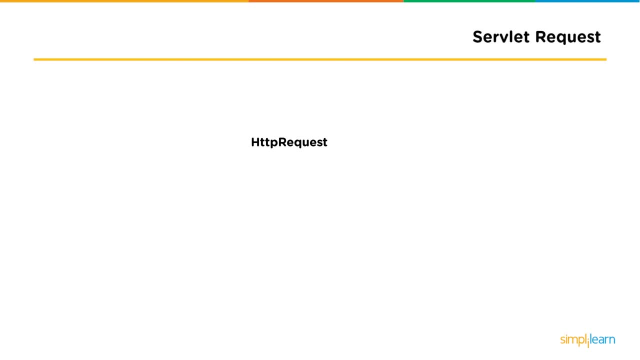 the request phase. in request, we have various types. the first one is being the http request. the http object is used to represent the http request to a browser that the user sends to the web application. thus, anything the browser sends is accessible through the http request, followed by the http request. 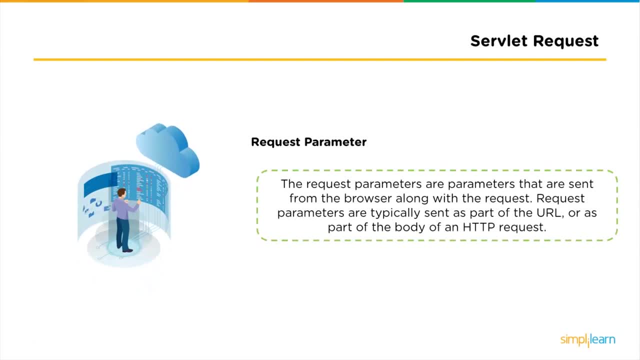 we have the request parameter. the request parameters are the parameters that are sent from the web browser along with the request. the request parameters are typically sent as a part of the url or as a part of the body of an http request, followed by the request parameter. we have the request header. the request headers are the name value pairs sent by the. 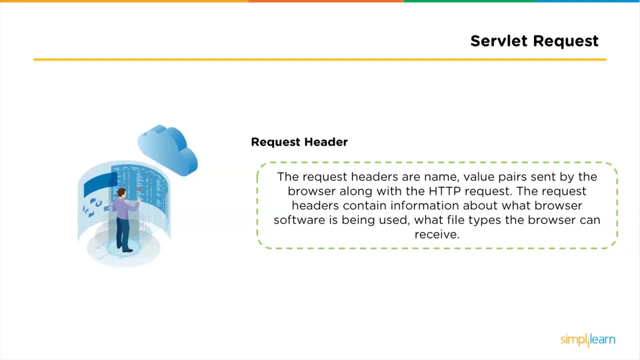 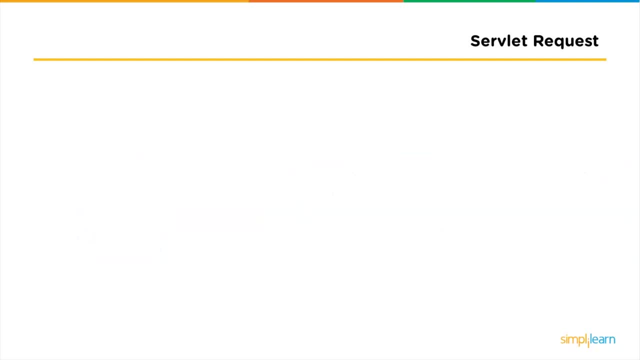 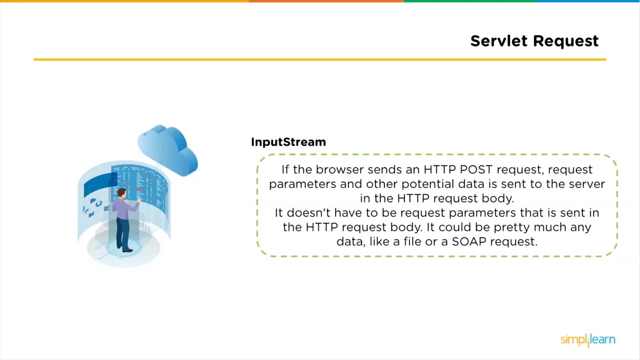 browser. along with the http request, the request headers contain the information about the web browser software being used, what type of files that the web browser can receive, etc. followed by the request header, we have the input string if the browser sends an http post request request parameters and. 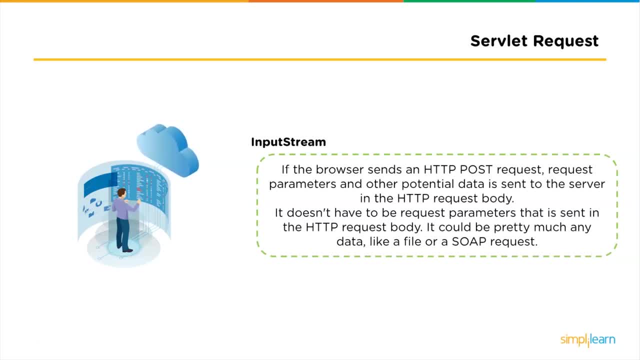 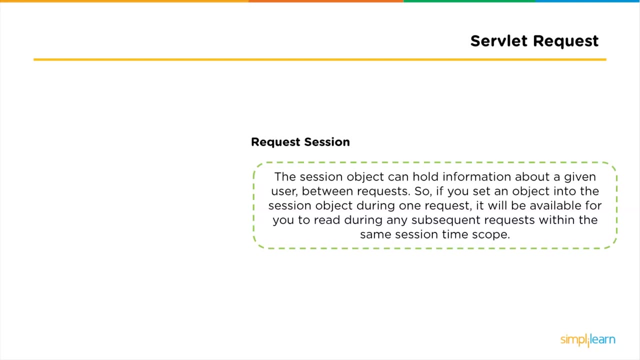 other potential data is sent to the server in the http request body, it doesn't have the request parameters. that is sent in http request body it could be pretty much as the data like file or soap request. the next one is a request session. the session object can hold information. 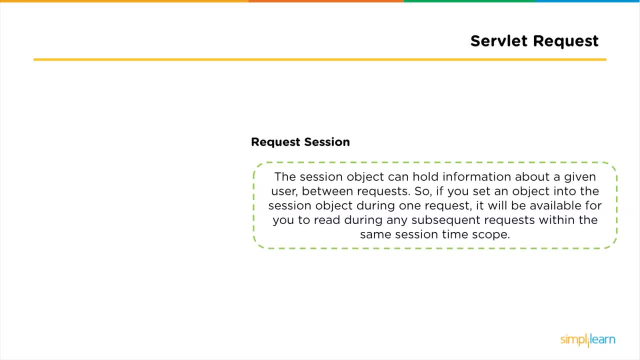 about a given user between the request. so if we have set an object into the session object during one request, it will be available for you to read during any subsequent request within the same session time scope followed by the request session. we have the servlet context, the servlet. 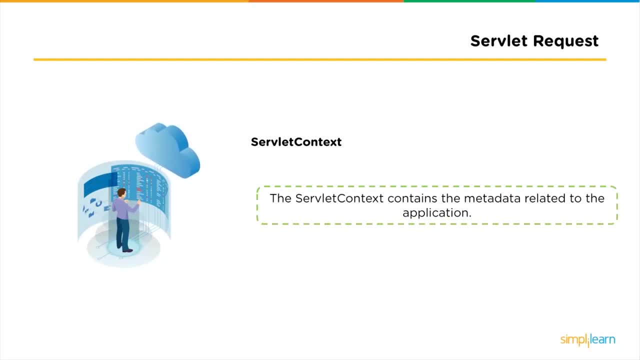 context contains the metadata related to the application, followed by servlet context. we will enter the response phase. in the response phase, we will deal with the first one, which is the http response. the http response is slightly different than the new request response. response is somewhat similar to the previous one, but it is a little different from the 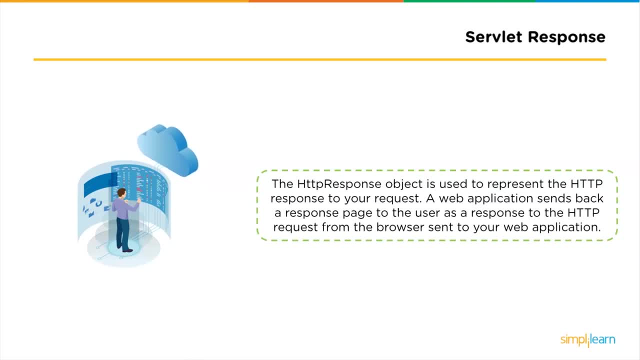 previous one. it is relatively similar. the next two is the activity, which is the set up of the. The HTTP response object is used to represent the HTTP response to your request. A web application sends back a response page to the user as a response to the HTTP request. 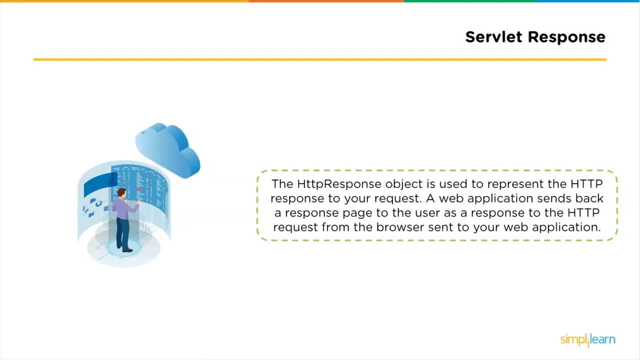 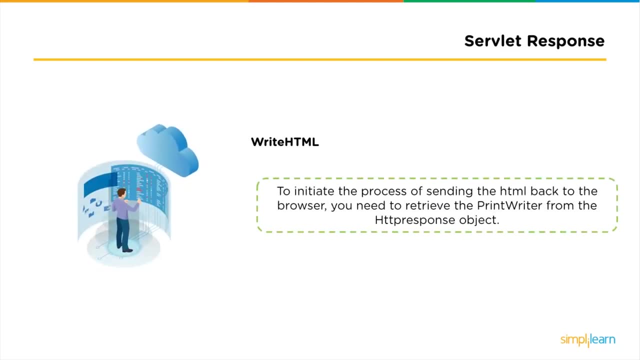 from the browser sent to your web application, Followed by the HTTP response. we have the writeHTML. To initiate the process of sending the HTML back to the browser, you need to retrieve the printWriter from the HTTP response object. This can be done using the writeHTML. 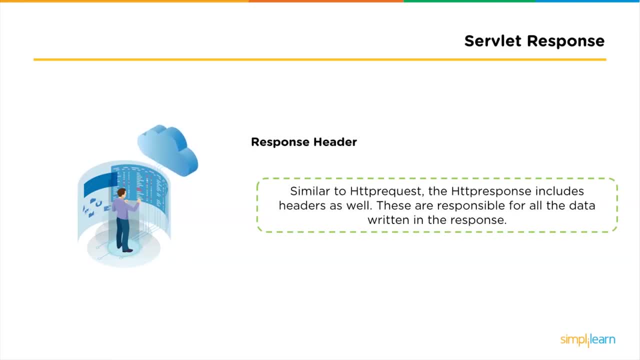 Followed by the writeHTML. we have the response header. Similar to HTTP request, the HTTP response includes headers as well. These are responsible for all the data written in the response, Followed by response header. we have content type. The content type header is responsible to tell the browser about the type of content. 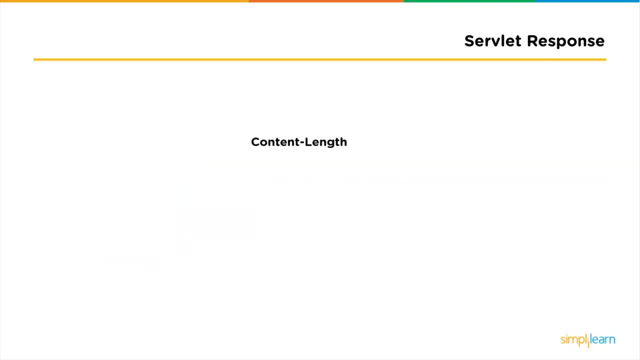 you are sending in the return, Followed by content type. we have the content length. The content length header is responsible for telling you about the number of bytes your servlet is sending you in return, Followed by the writeHTML, Followed by content length. we have redirection. 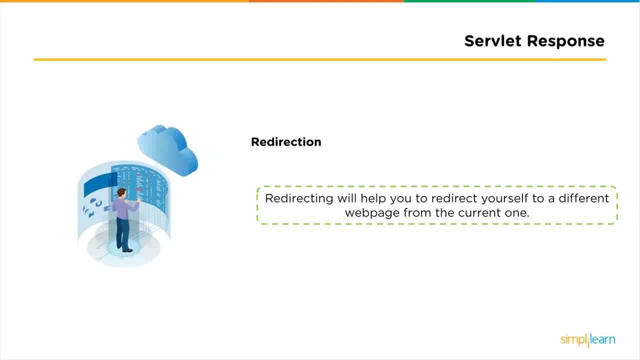 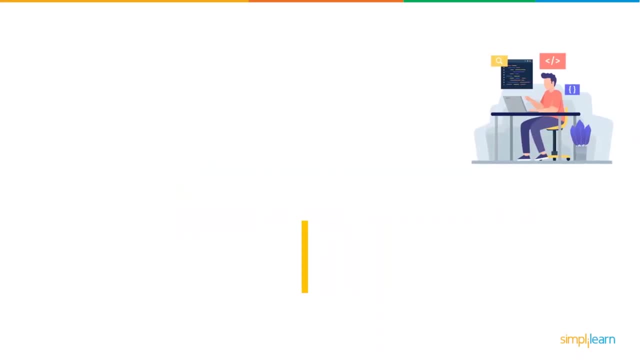 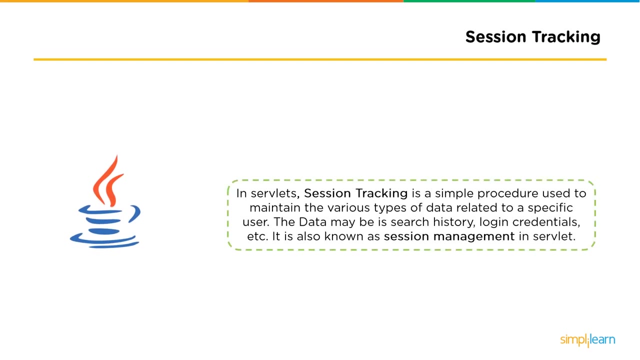 Redirecting will help you to redirect yourself to the different web pages from the current one. So these were the HTTP requests and responses in Java servlets. Now we will enter the next part where we will deal with the session tracking and cookies. So first we will understand session tracking. 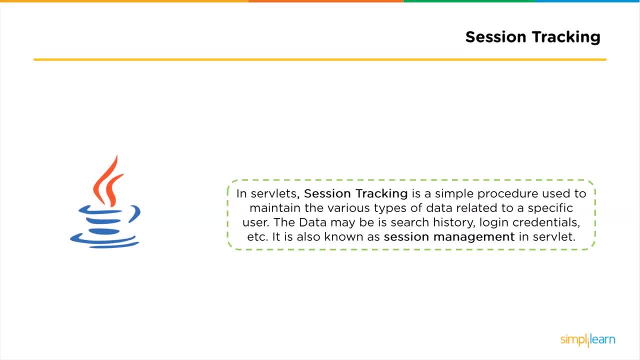 Session simply means a particular time of interval. Session tracking is a way to maintain state or data belonging to a user. It is also known as session management in servlets. HTTP protocol is stateless, so we need to maintain state using session tracking techniques. 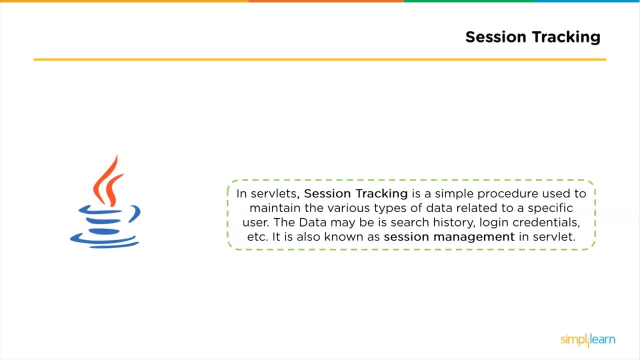 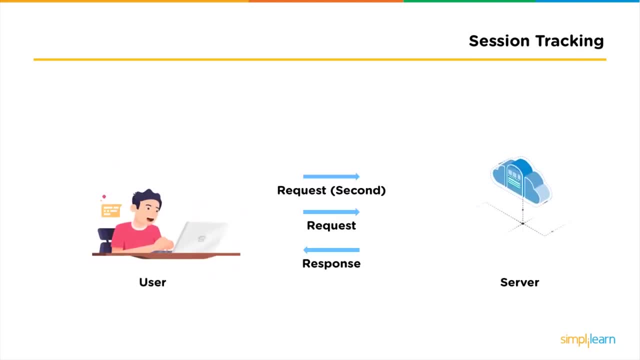 Each time the user requests to the server, the server treats the request as a new request. So we need to maintain the state of a user to recognize a particular user. You can understand this in a better way by looking at the picture shown on the presentation. 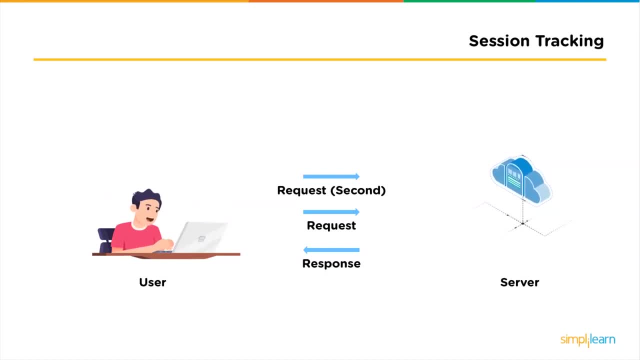 Each time you send a request, you will be receiving a response from the server, as well as this particular request. This particular request will be recorded as a state in order to recognize you as a particular user. Now, after session tracking, we will enter into cookies. 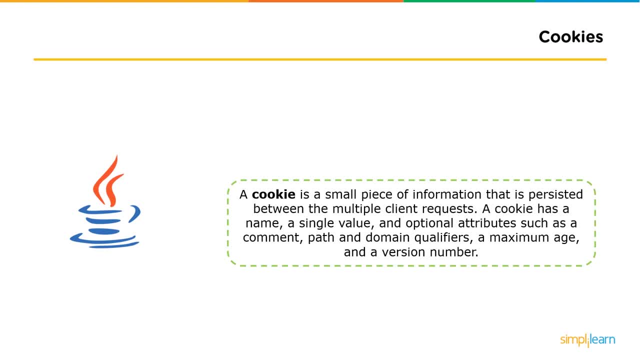 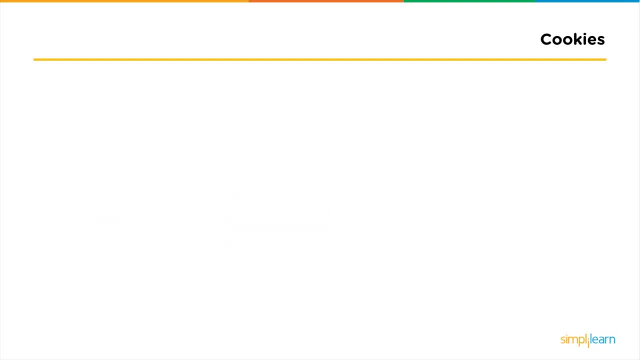 Cookie is a small piece of information that is persisted between multiple client requests. A cookie has a name, a single value and optional attributes such as comment path and domain qualifiers, a maximum age and a version number. By default, each request is considered as a new request. 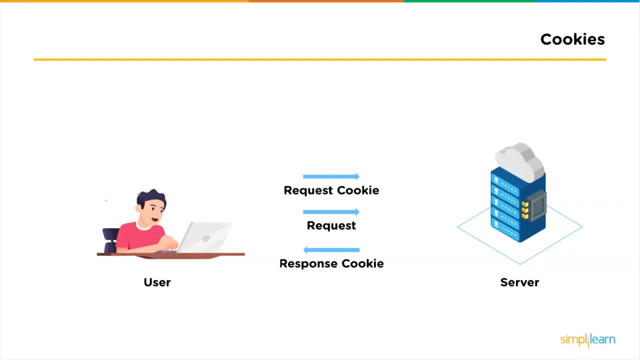 In cookie technique we add a cookie with response from the servlet, So cookie is stored in cache of a browser. After that, if the request is sent by the user, the cookie is added with a request by default. Thus we recognize the user as an old user. 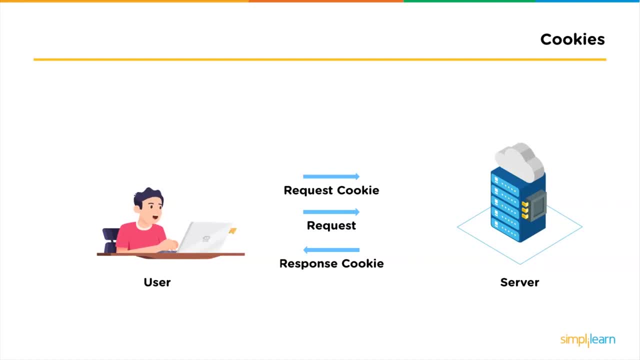 There are two types of cookies. They are non-persistent cookie and persistent cookie. Let's understand non-persistent cookie first. A non-persistent cookie is valid for a single session only. It is removed each time when the user closes the browser. 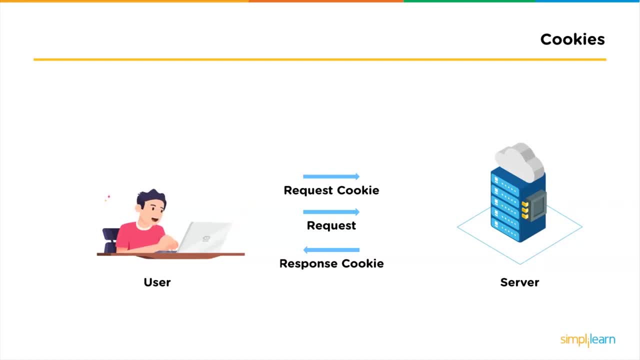 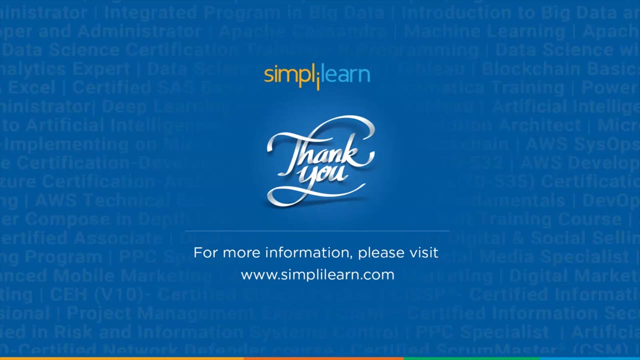 Now let us understand the persistent cookie. The persistent cookie is valid for multiple sessions. It is not removed each time when the user closes the browser. It is only removed when the user logs out or signs out from the browser. So with this we have come to an end of Java servlets tutorial.